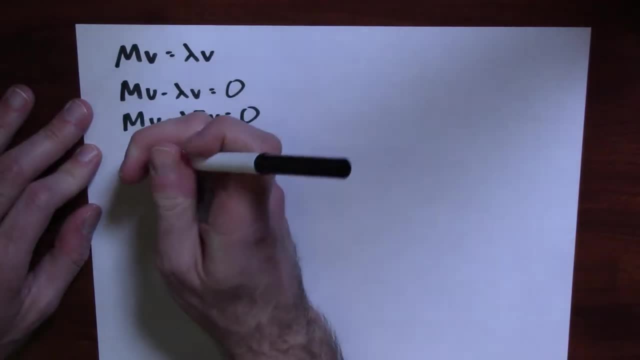 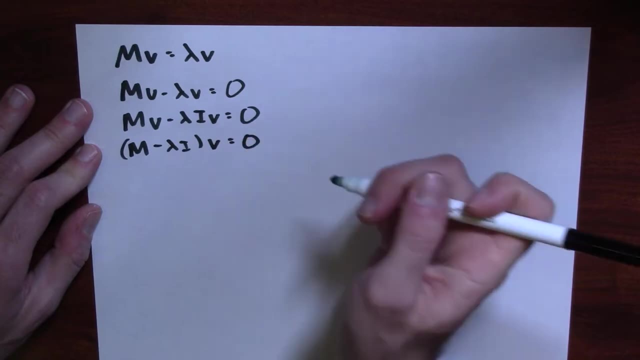 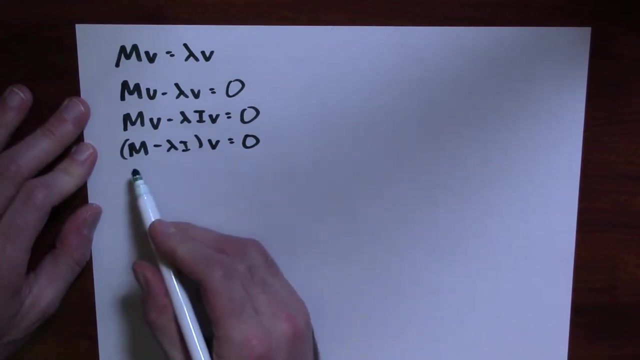 Then I could factor out a common vector v here And I could write this as m minus lambda v. lambda times the identity times. the vector v equals the zero vector. Now, what's important about this is that I've got a non-trivial vector v. 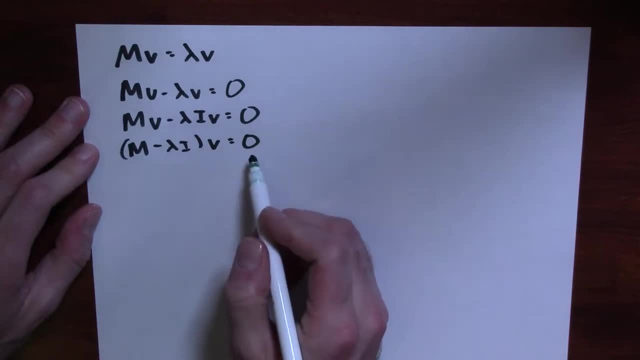 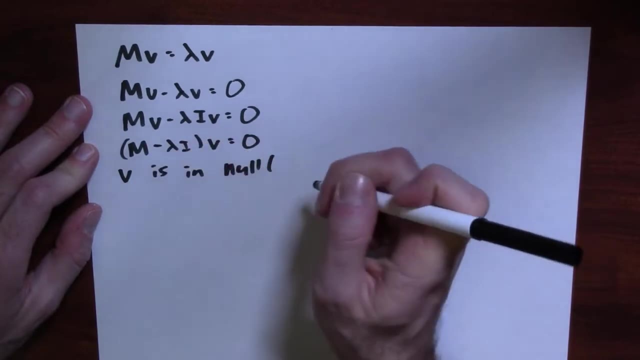 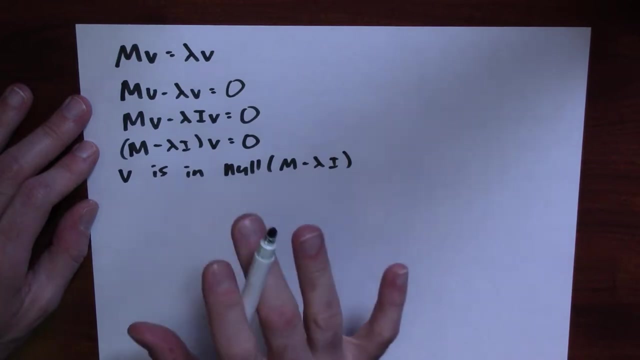 which I've multiplied by m minus lambda times the identity and I'm getting the zero vector. What this means is that v is some non-trivial vector in the null space or the kernel of m minus lambda times the identity. v is a non-trivial element of this null space or this kernel. 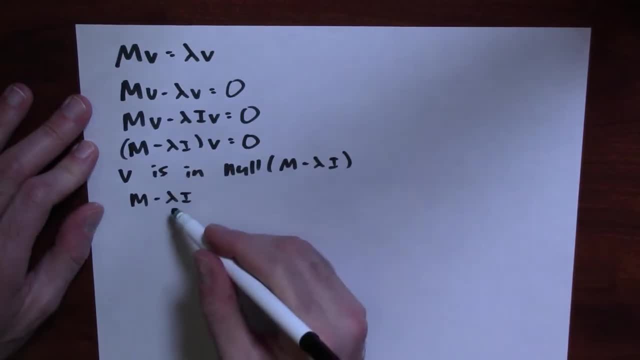 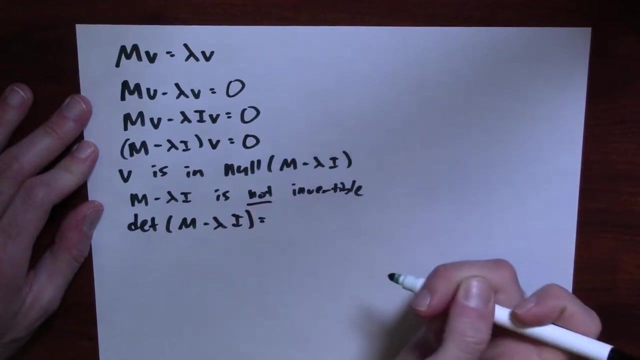 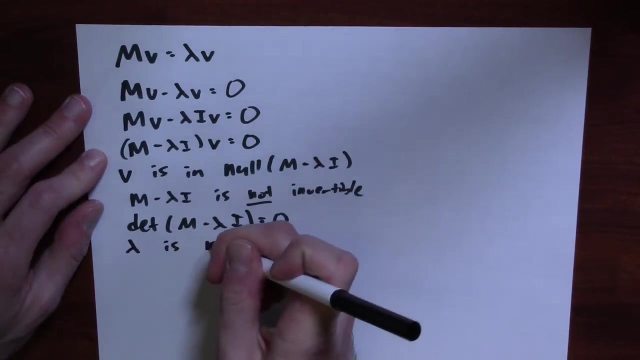 That means that m minus lambda times the identity for this eigenvalue, lambda is not invertible. And because it's not invertible, that tells me that the determinant of m minus lambda times the identity must be equal to the number zero. Or in other words, it's telling me that lambda is a root. 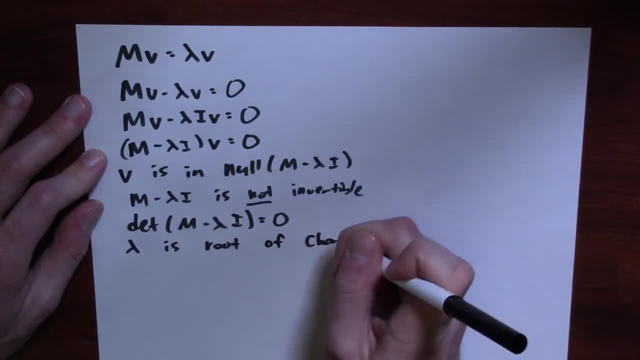 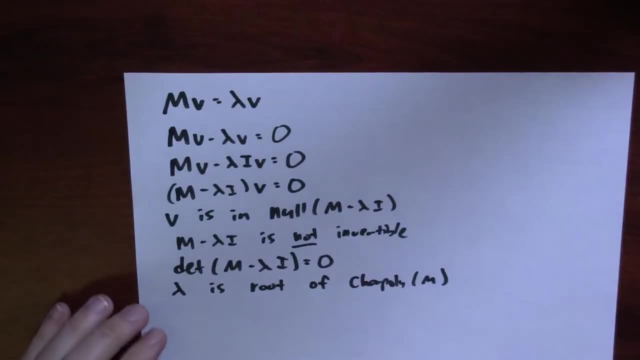 lambda is a root of the characteristic polynomial of this matrix m, And this argument can be reversed. What I mean is that I can run this argument exactly backwards. I can start at the bottom and end up at the top. I can begin with lambda being some root of the characteristic polynomial of this square matrix m. 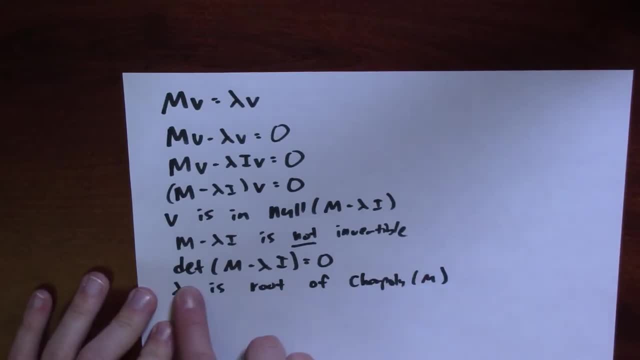 and lambda being a root of that characteristic polynomial, means that the determinant of m minus lambda times the identity matrix. this determinant vanishes If this determinant is equal to zero. that means that this matrix is not invertible. But this is a square matrix which isn't invertible. 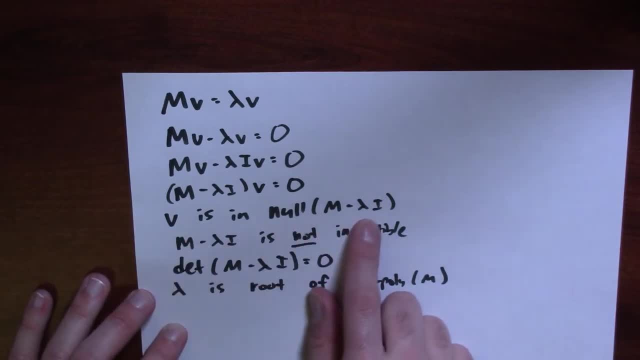 That means I can find some non-trivial vector v in its null space. That means that I can find a solution to this equation: for some non-zero vector v, m minus lambda times, the identity times, the vector v is the zero vector. But then just expanding this out and rearranging I can find a non-trivial solution to this equation. 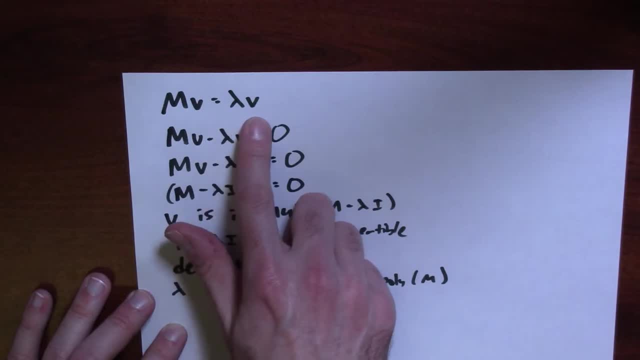 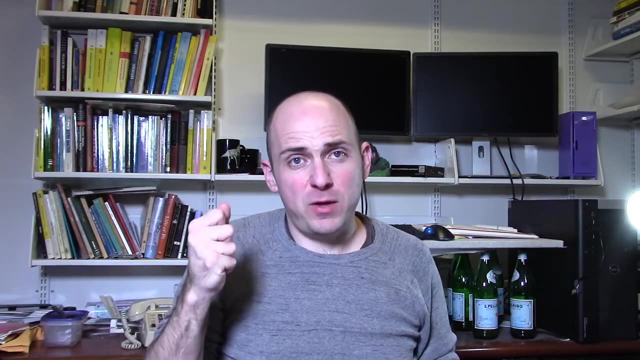 The matrix times. the vector v is lambda times v And this lambda started out life as a root of the characteristic polynomial of m. So if I start with the root of the characteristic polynomial, I get an eigenvalue, And if I start with an eigenvalue, I get a root of the characteristic polynomial.